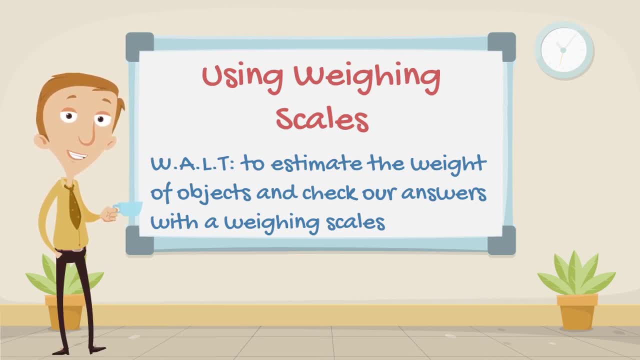 Hello and welcome back to Wrongmar. In today's maths lesson we're taking a look at using weighing scales. Our wall for today is to estimate the weight of objects and to check our answers with a weighing scales. But first let's warm up. I'm going to show you a picture of an object. 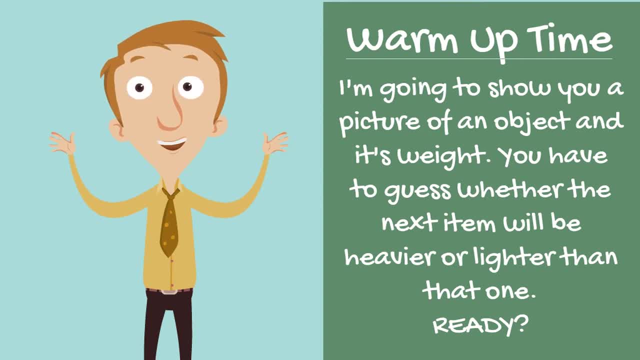 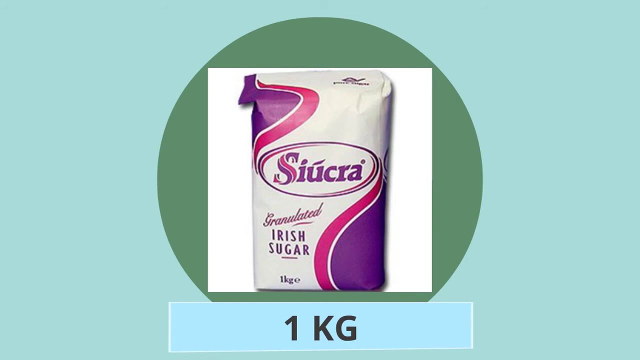 and its weight. You have to guess whether the next item is going to be heavier or lighter than that one. I'll show you the first picture to get you started. So here is our bag of sugar. It weighs one kilogram. Do you think the next picture is going to be heavier or lighter than this bag of? 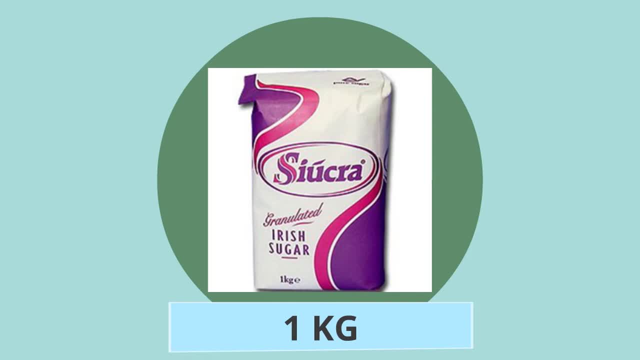 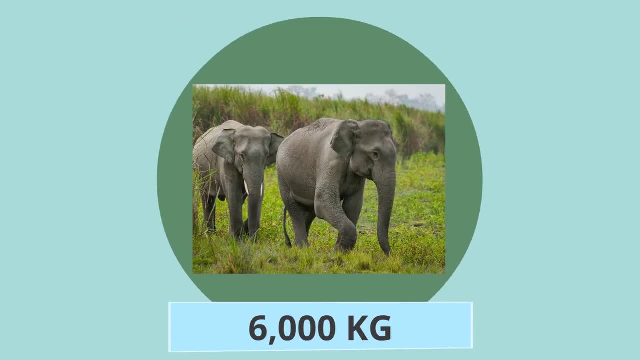 sugar. Pause the video and write down your answer. Well, it is an elephant, and an African elephant as well, which is the heaviest of all. This is 6,000 kilograms, so it is definitely heavier than a bag of sugar. What about the next? 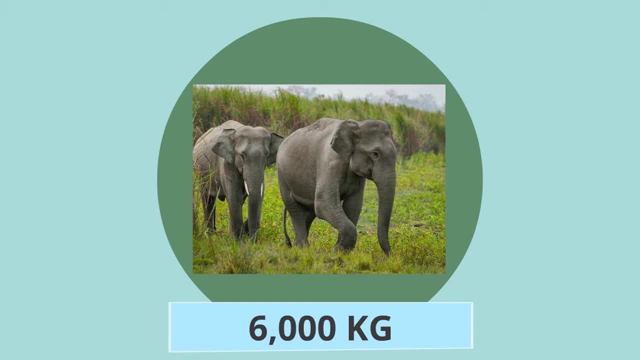 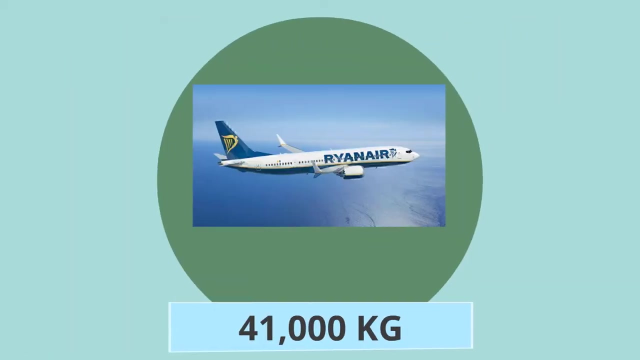 item. Do you think it's going to be heavier or lighter than this elephant? Pause the video and write down your answer. Well, our next item is a Boeing 747 airplane which weighs a huge 41,000 kilograms, So it is definitely heavier than an elephant. What about the next one? Do you think it's? 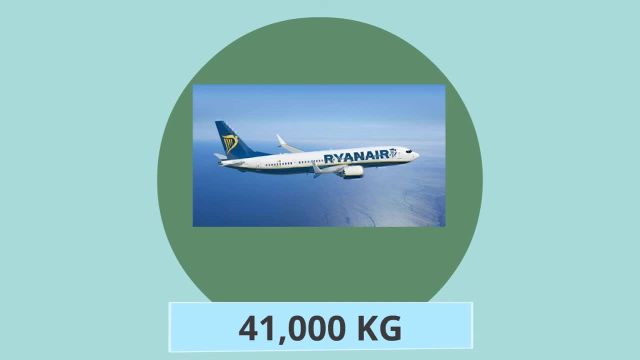 going to be heavier or lighter than this Boeing 747?? Pause the video and write down your answer. Well, our next picture is a blackbird, and a blackbird only weighs 100 grams, so it is much lighter than our airplane. What about our next picture? Do you think it's going to be heavier or 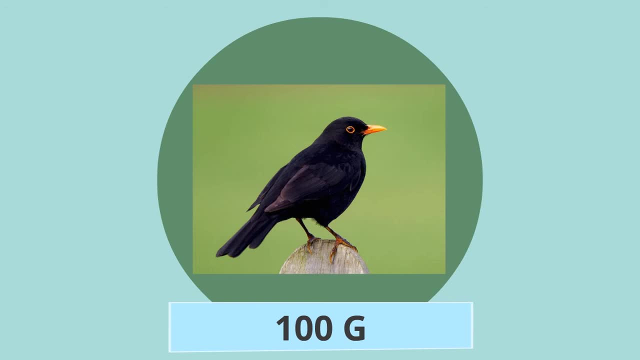 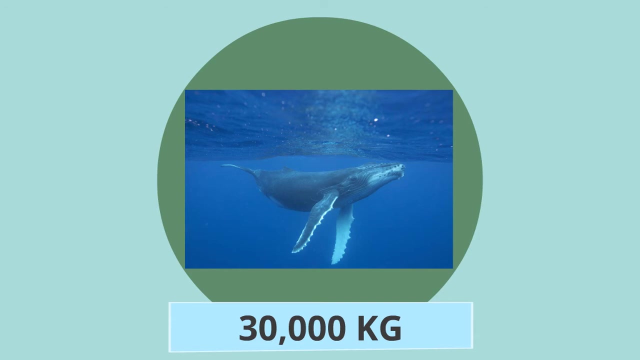 lighter than this blackbird. Pause the video and write down your answer. Well, our next picture is a humpback whale which weighs 30,000 kilograms, nearly as much as the plane. So it's definitely heavier than the blackbird. What about our next picture, Our last one? Do you think it's going to? 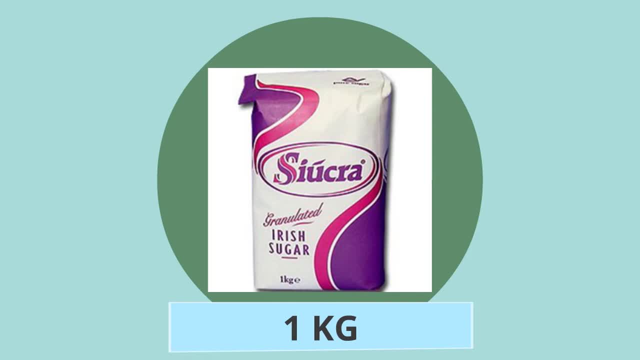 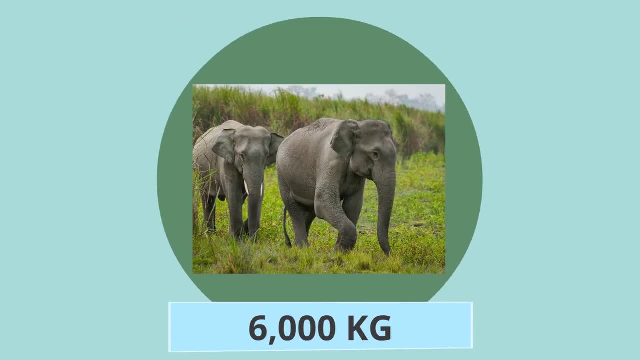 sugar. Pause the video and write down your answer. Well, it is an elephant, and an African elephant as well, which is the heaviest of all. This is 6,000 kilograms, so it is definitely heavier than a bag of sugar. What about the next? 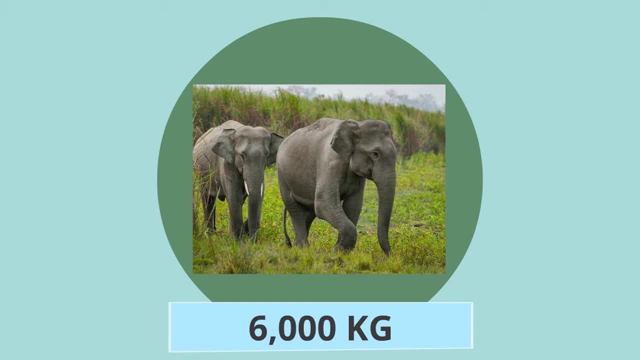 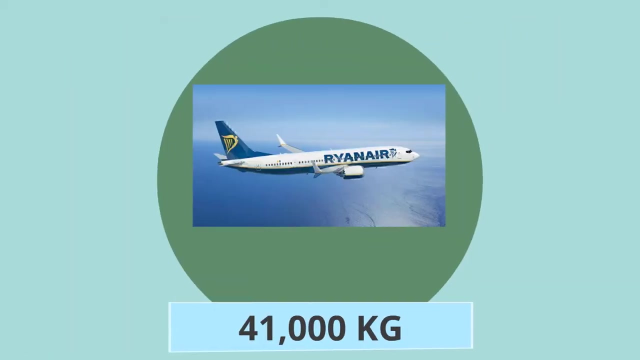 item. Do you think it's going to be heavier or lighter than this elephant? Pause the video and write down your answer. Well, our next item is a Boeing 747 airplane which weighs a huge 41,000 kilograms, So it is definitely heavier than an elephant. What about the next one? Do you think it's? 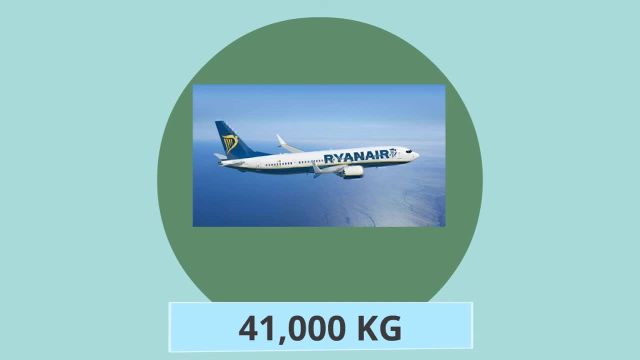 going to be heavier or lighter than this Boeing 747?? Pause the video and write down your answer. Well, our next picture is a blackbird, and a blackbird only weighs 100 grams, so it is much lighter than our airplane. What about our next picture? Do you think it's going to be heavier or 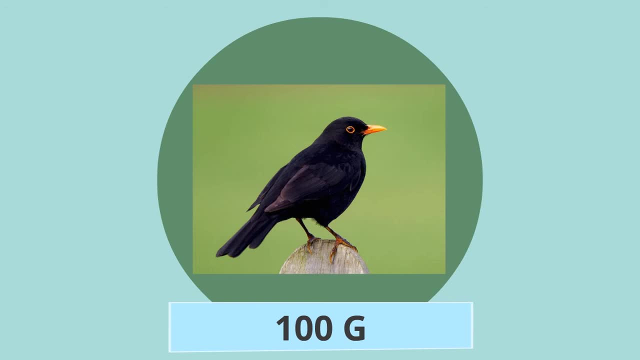 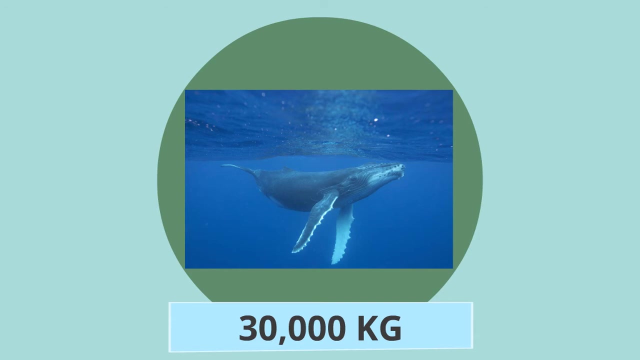 lighter than this blackbird. Pause the video and write down your answer. Well, our next picture is a humpback whale which weighs 30,000 kilograms, nearly as much as the plane. So it's definitely heavier than the blackbird. What about our next picture, Our last one? Do you think it's going to? 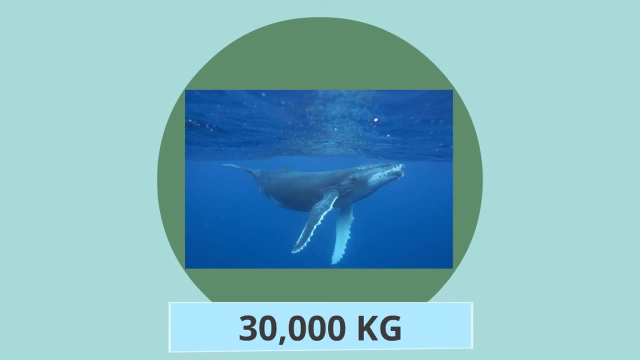 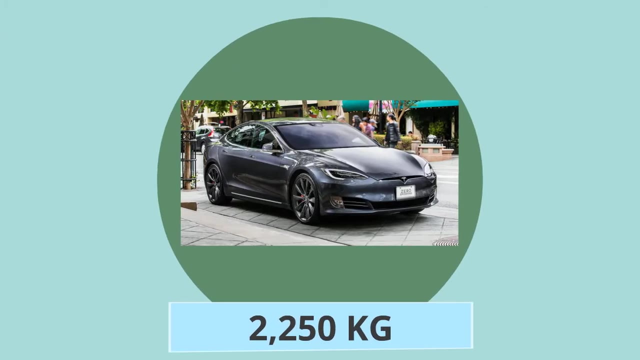 be heavier or lighter. Pause the video and write down your answer. Well, our next picture is a Tesla Model S, which only weighs 2,250 kg, So it is much lighter than a humpback whale. Great, We are all warmed up and ready to jump into our lesson. For our last lesson, we learned that 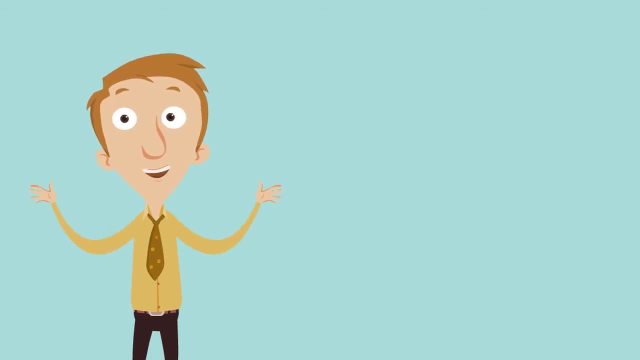 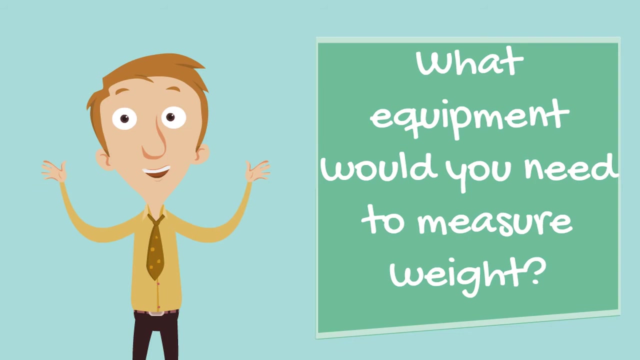 there are different units of measurement for when we are measuring, So let's take a look at our measuring weight. But what equipment do you think we would need to use to measure weight? You might remember that when we were talking about length, we mentioned things like rulers and measuring. 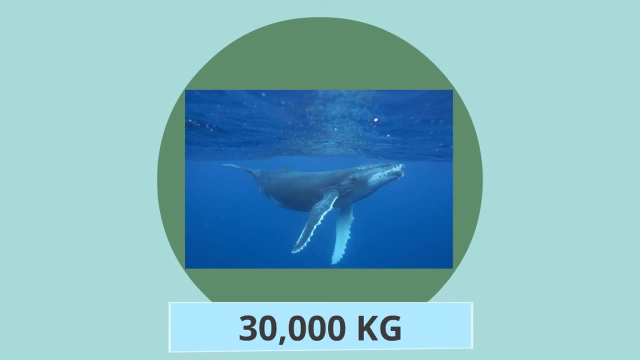 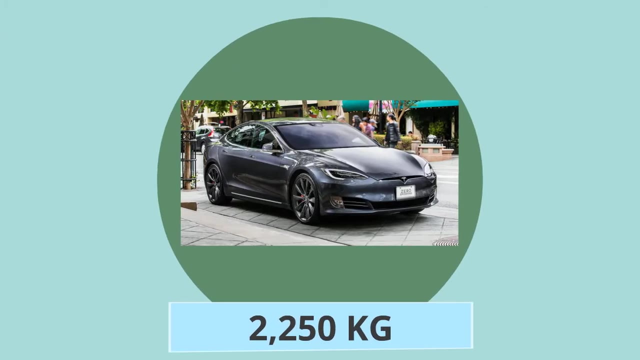 be heavier or lighter. Pause the video and write down your answer. Well, our next picture is a Tesla Model S, which only weighs 2,250 kg, So it is much lighter than a humpback whale. Great, We are all warmed up and ready to jump into our lesson. For our last lesson, we learned that 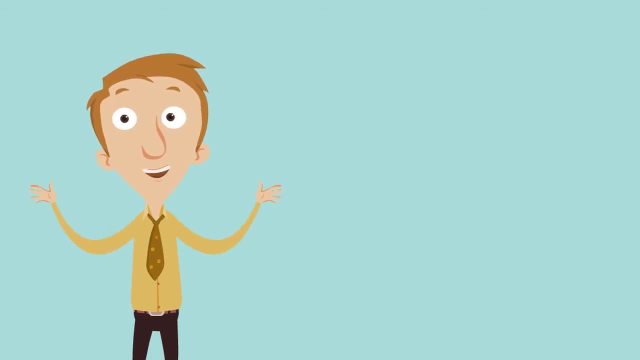 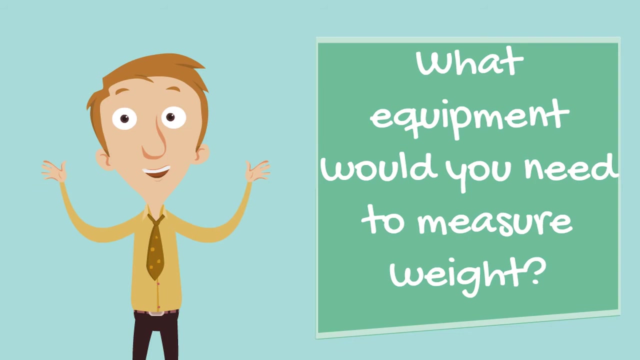 there are different units of measurement for when we are measuring, So let's take a look at our measuring weight. But what equipment do you think we would need to use to measure weight? You might remember that when we were talking about length, we mentioned things like rulers and measuring. 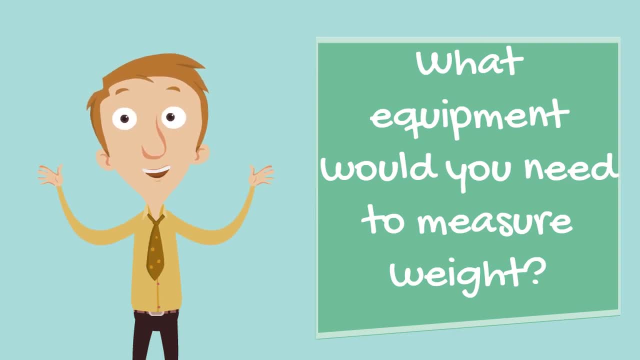 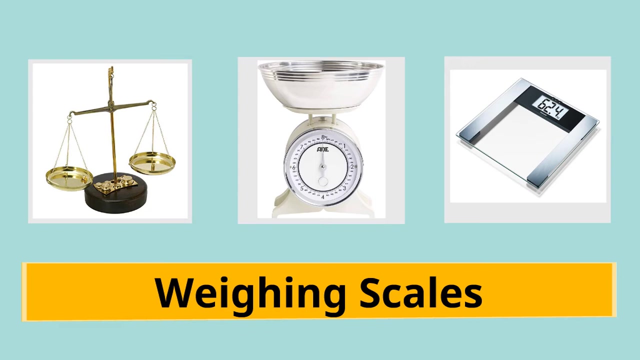 tapes, But what do we use when we want to measure weight? Pause the video and write down an answer. Well, the piece of equipment that we use is called a weighing scales, But there are three different types of weighing scales that we use to measure weight. So let's take a look at our. 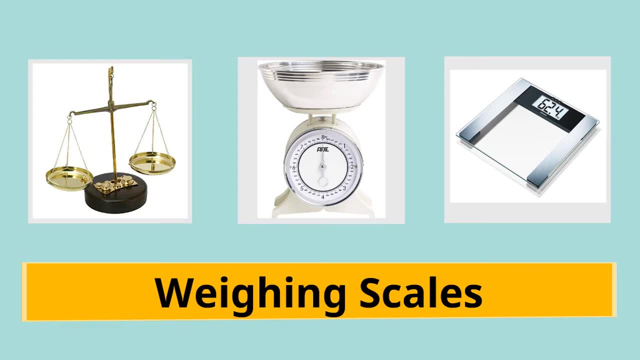 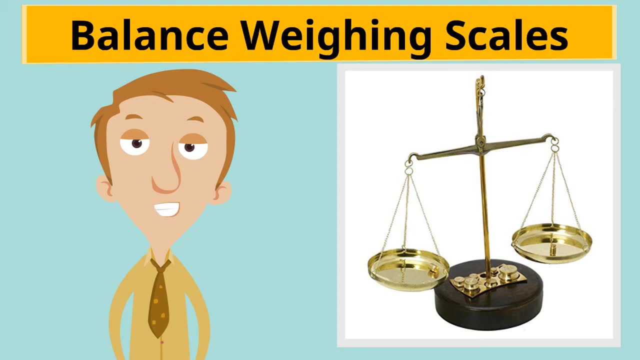 scales. The first one is called a balance weighing scales. It looks like this. They're quite old fashioned and rare these days, So maybe if you've got a granny who bakes a lot or a granddad who likes to bake, they might have one of these stashed away somewhere. The other type of weighing scales: 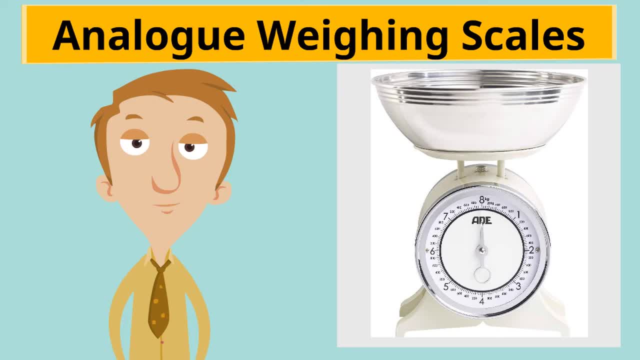 that you've probably seen before is an analog weighing scales. It looks like this And you usually see them when you're weighing things in the kitchen or maybe in the bathroom on the floor, if it's an older weighing scales. The third and final weighing scales is probably the most. 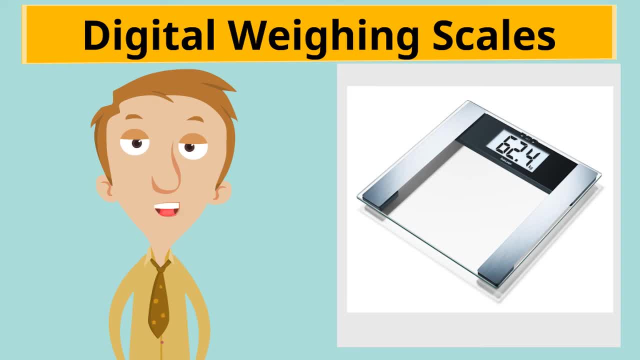 common one to see in shops now. That is, a digital weighing scales. You'll see these if you're in the supermarket and you need to weigh out some vegetables or fruit, And if you do a lot of baking at home, you might also get some on your desk. But I'm going to show you a little bit more of this at. 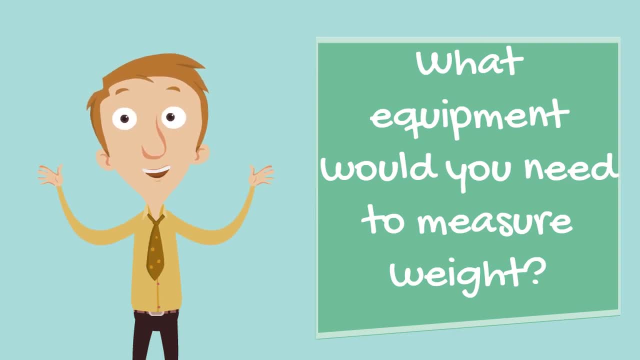 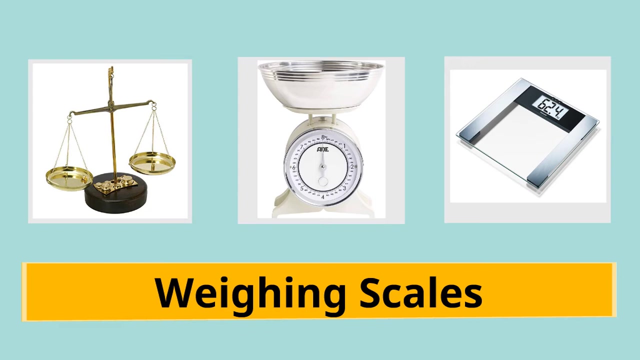 tapes, But what do we use when we want to measure weight? Pause the video and write down an answer. Well, the piece of equipment that we use is called a weighing scales, But there are three different types of weighing scales that we use to measure weight. So let's take a look at our. 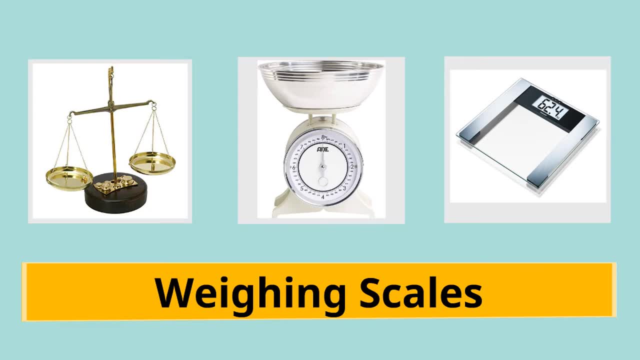 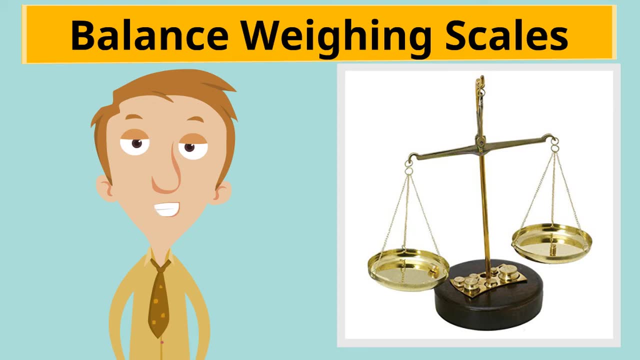 scales. The first one is called a balance weighing scales. It looks like this. They're quite old fashioned and rare these days, So maybe if you've got a granny who bakes a lot or a granddad who likes to bake, they might have one of these stashed away somewhere. The other type of weighing scales: 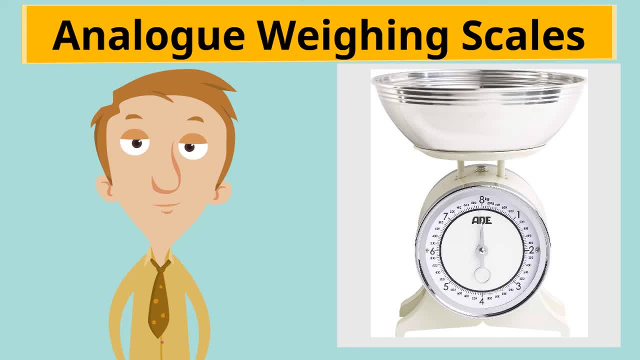 that you've probably seen before is an analog weighing scales. It looks like this And you usually see them when you're weighing things in the kitchen or maybe in the bathroom on the floor, if it's an older weighing scales. The third and final weighing scales is probably the 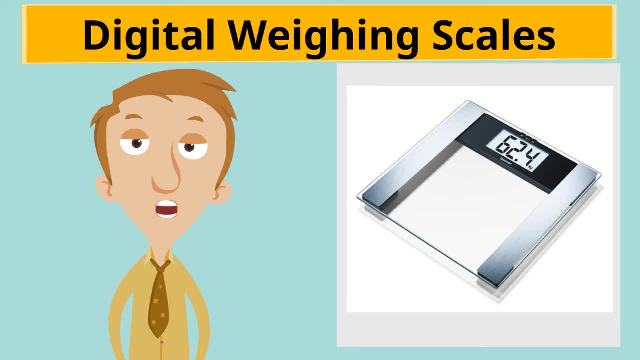 most common one to see in shops. now, That is, a digital weighing scales. You'll see these if you're in the supermarket and you need to weigh out some vegetables or fruit, And if you do a lot of baking at home, you might also see a small scale that you might want to measure. So let's take a. 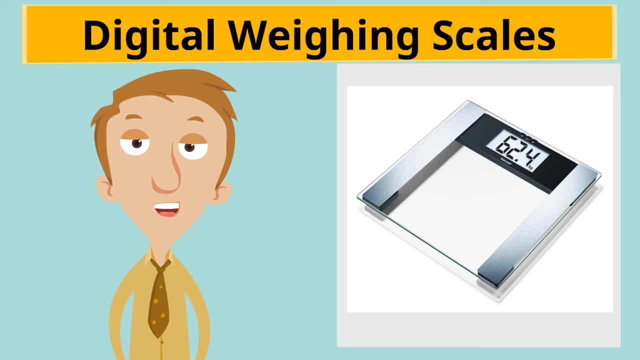 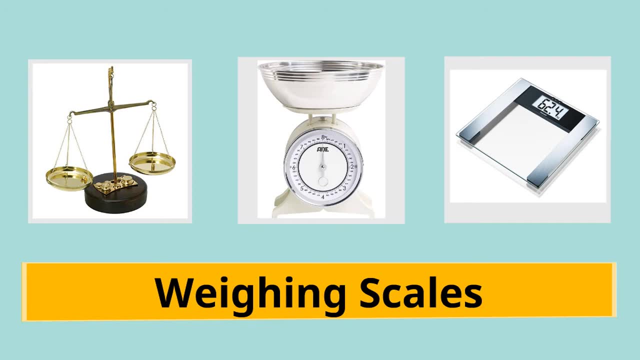 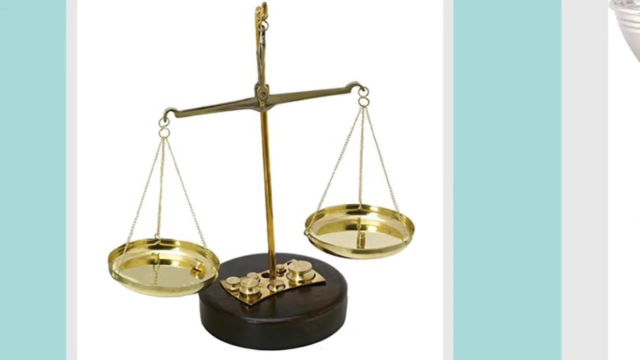 have one of these in your kitchen, because they're very quick and very handy. The way that we read and use these three different types of weighing scales are all a little bit different from one another, so let's take a closer look at the balance scale first. Balance scale works exactly the same way as a seesaw. 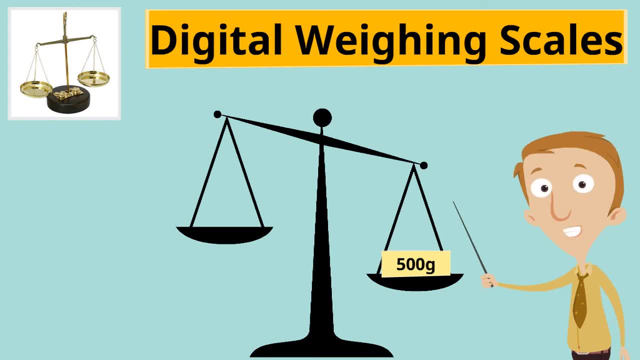 if you've ever been on one of them. On one side of the scale you put the weight that you want to measure out like this: 500 grams. To balance the scales, you'll need to put an object with the equal weight on the other end. so say we were. 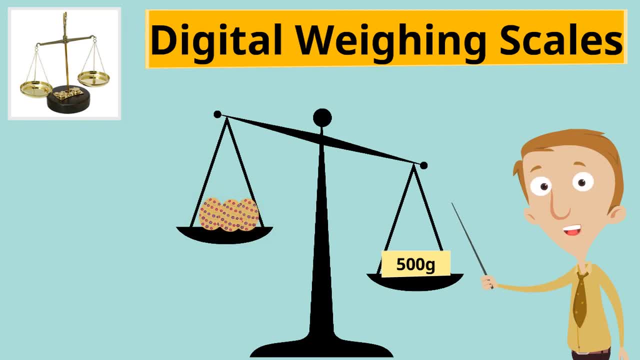 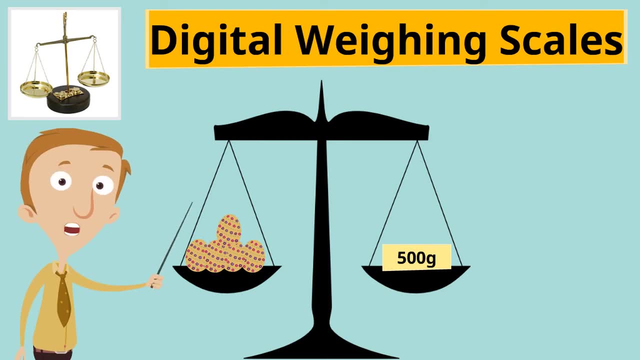 measuring eggs. we need to keep on putting eggs on until it was flat and balanced. Then we know we have 500 grams of eggs. So we always want both sides of the weighing scale to be the same. Now that you know that, let's. 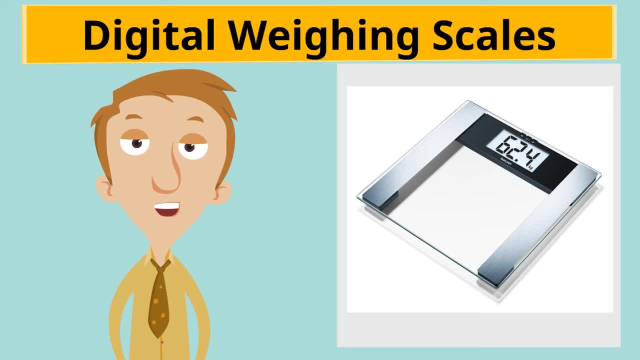 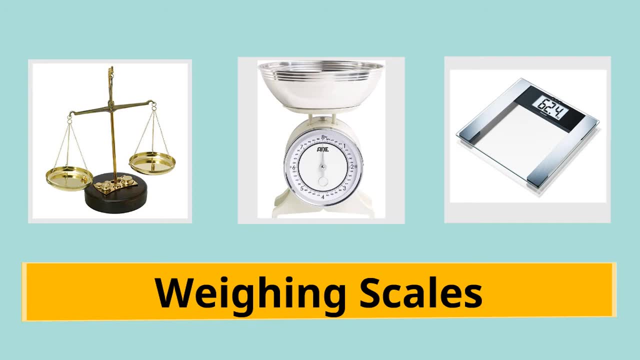 home. In the other hand, we have a digital weighing scale, so we're going to take this and, let's see, also have one of these in your kitchen, because they're very quick and very handy. The way that we read and use these three different types of weighing scales are all a little bit different. 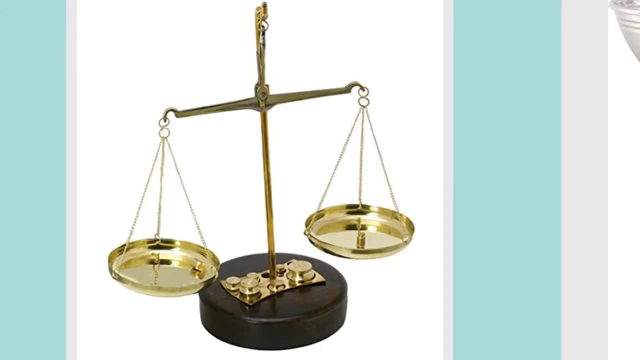 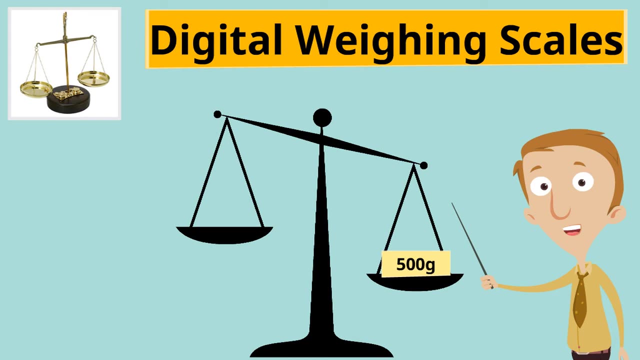 from one another. So let's take a closer look at the balance scale first. A balance scale works exactly the same way as a seesaw- if you've ever been on one of them. On one side of the scale you put the weight that you want to measure out, like this, 500 grams, To balance the scales. 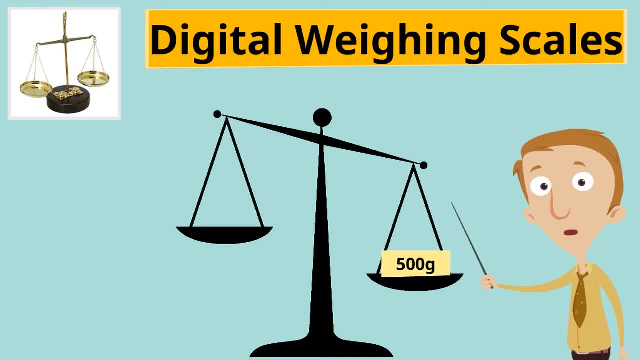 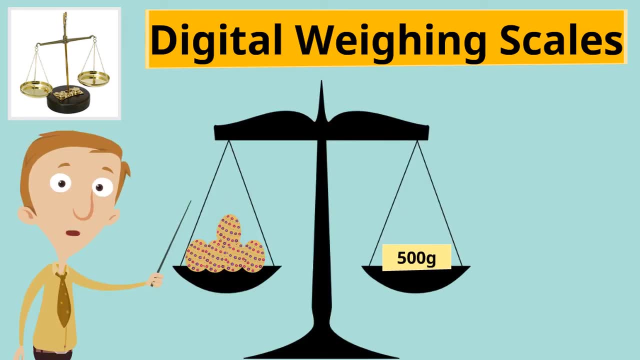 you'll need to put an object with the equal weight on the other end. So say we were measuring eggs. we need to keep on putting eggs on until it was flat and balanced. Then we know we have 500 grams of eggs. So we always want both sides of the weighing scale to be the same. 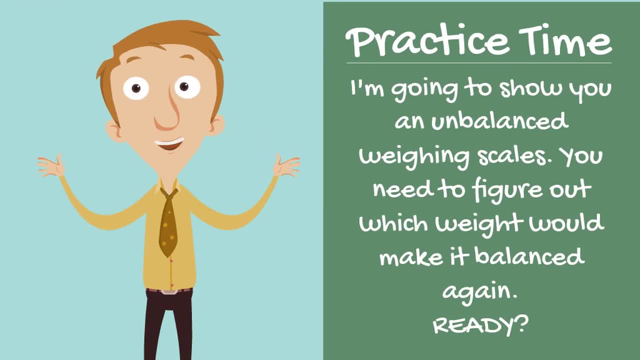 Now, just to make sure that you're understanding what I'm saying, let's take a closer look at the balance scale. So, let's take a closer look at the balance scale. So let's take a closer look at the How did you know that? Let's practice a few scale questions? I'm going to show you an unbalanced. 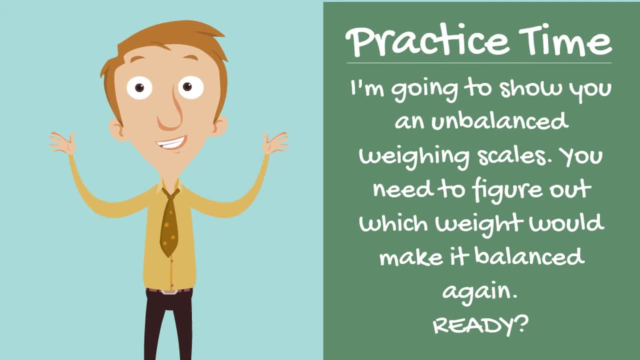 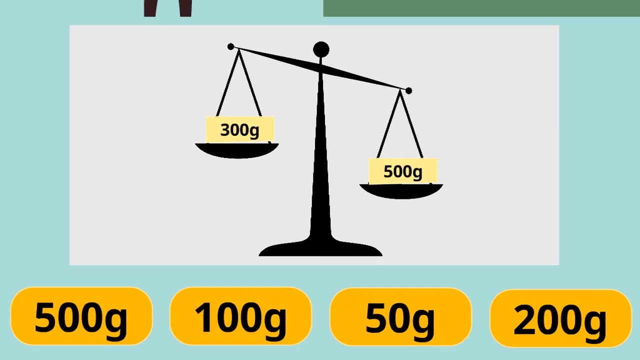 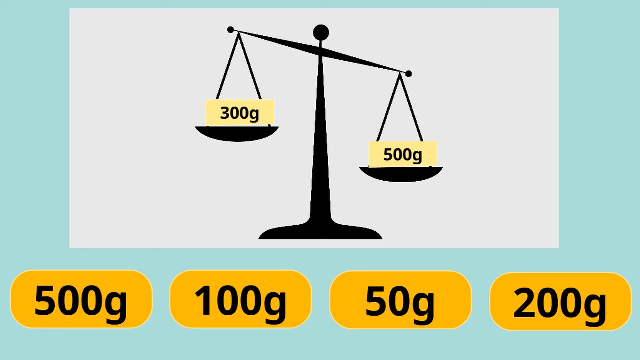 weighing scale. You need to figure out what weight you would put on the other side to make it balanced again. You ready? Okay, take a look at this weighing scales. So on one side we have got 500 grams and on the other side we've already got 300, but we need to add another weight to balance it out, Can you? figure out what weight you would put on the other side to make it balanced again. So let's take a closer look at this weighing scale. You need to figure out what weight you would put on the other side to make it balanced again. Can you figure out what weight you would put on the other side to make it balanced again? So let's take a closer look at this weighing scale. You need to figure out what weight you would 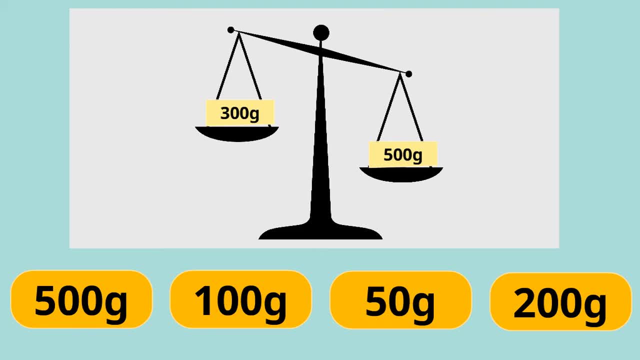 Pause the video and write down your answer. Well, to balance this weighing scales out, we'd need to add another 200 grams to this side, so that both of the sides are equal to 500 grams. Did you get that? Let's try another one. Have a look at this. 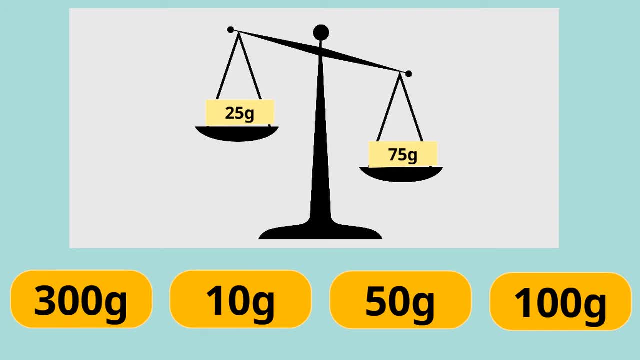 weighing scales. One side is 75 grams, The other side is 25 grams, Which one needs a register? 100. 500 grams. 70. 50 הדс. 100. 200.. of the weights down below, would we need to add to the 25 grams to make them even? 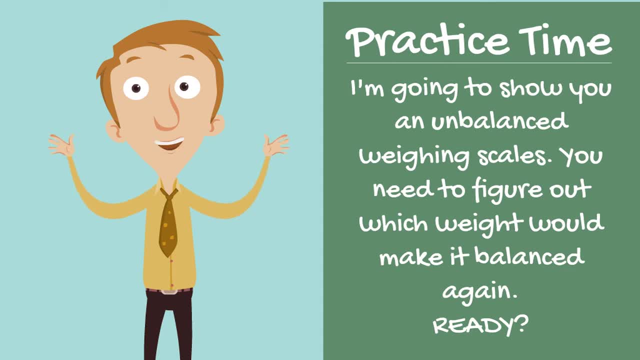 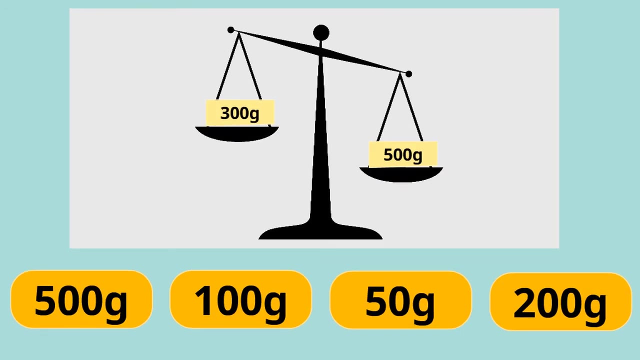 prove it right here, practice a few scale questions. I'm going to show you an unbalanced weighing scale. You need to figure out what weight you would put on the other side to make it balanced again. You ready? Okay, take a look at this weighing scales. So on one side we have got 500 grams and on the other side, 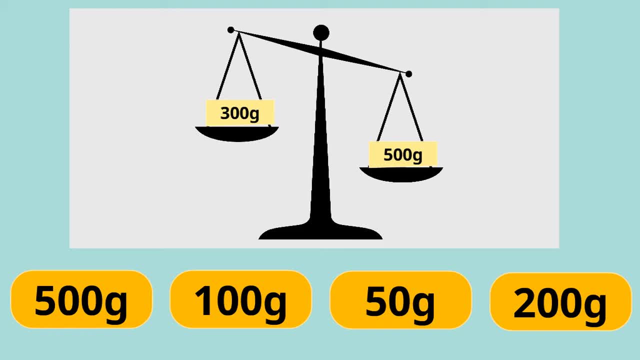 we've already got 300, but we need to add another weight to balance it out. Can you figure out which one of the weights it is? Pause the video and write down your answer. Well, to balance this weighing scales out, we'd need to add another 200 grams to this side. 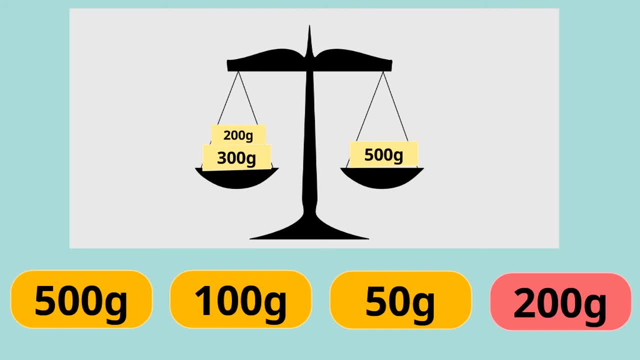 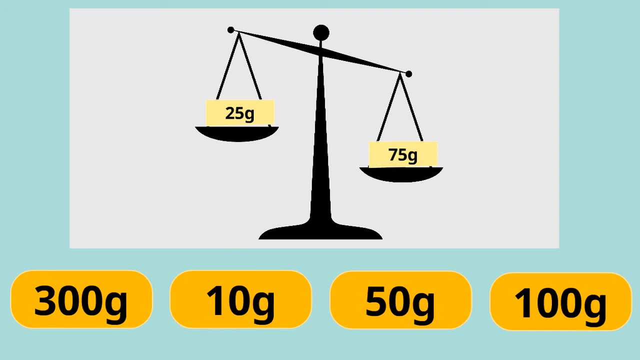 so that both of the sides are equal to 500 grams. Did you get that? Let's try another one. Have a look at this weighing scales: One side is 75 grams, the other side is 25 grams. Which one of the weights is the most important? 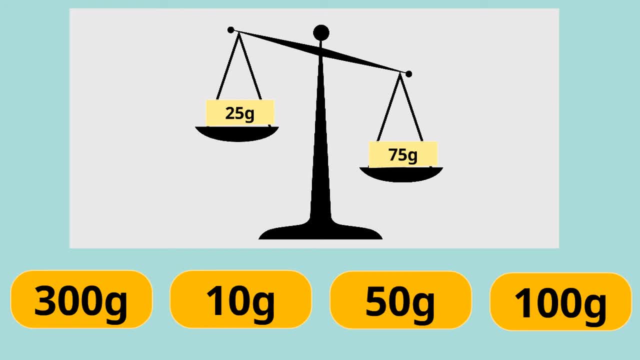 One of the weights down below. would we need to add to the 25 grams to make them even? Pause the video and write down your answer. Well, the answer is: we would need to add the 50 grams to this side to make sure that they're both. 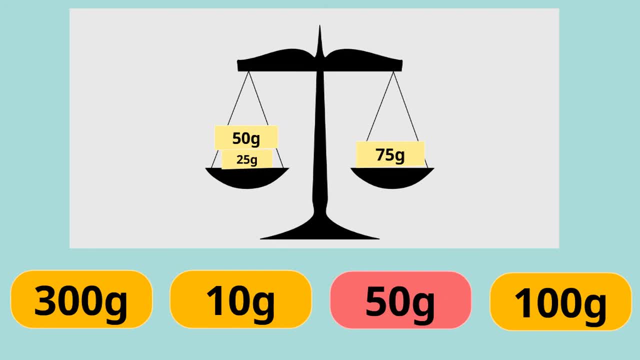 equal to 75.. 50 and 25 is 75, and the other side was already 75.. Let's try another one, slightly more difficult one this time. Let's take a look at this scale. So we've got 250 on one side and nothing on the other side. 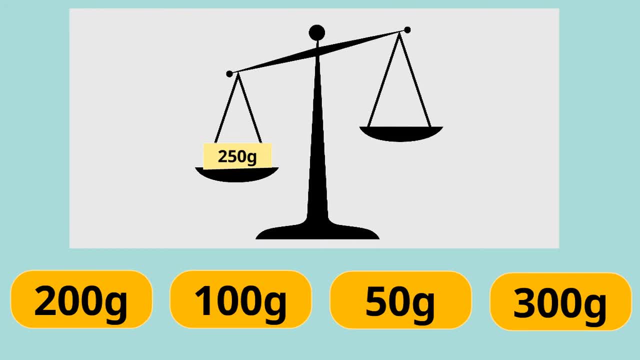 Which two weights would we need to add to the other side to make it equal? Pause the video and give it a try. Well, the two weights we would need are the 200 gram weight and the 50 gram weight. That will make the two sides equal. Let's go for one last practice one, and this is probably the most. 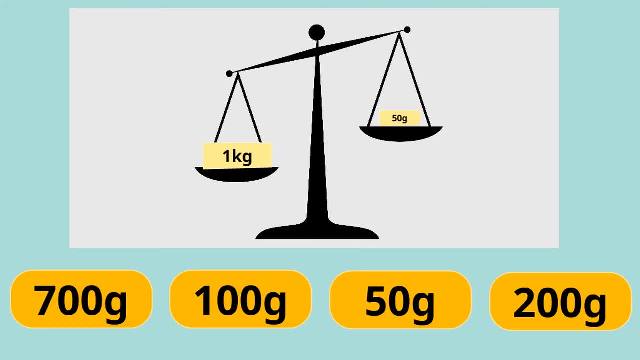 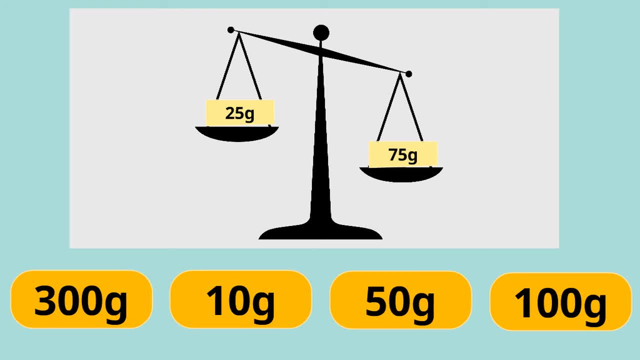 Pause the video and write down your answer. Well, the answer is: we would need to add the 50 grams to this side to make sure that they're both equal to 75.. 50 and 25 is 75 and the other side was already 75.. 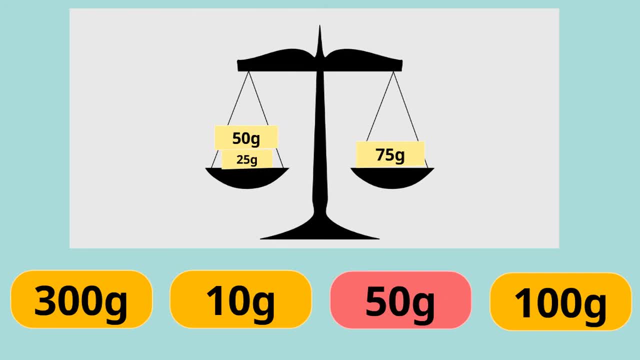 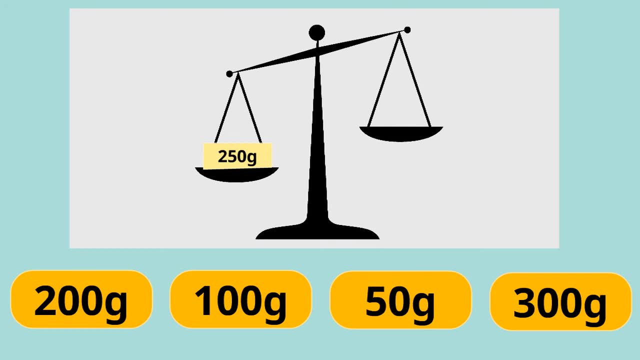 Let's try another one, a slightly more difficult one this time. Have a look at this scale. So we've got 250 on one side and nothing on the other side. Which two weights would we need to add to the other side to make it equal? Pause the. 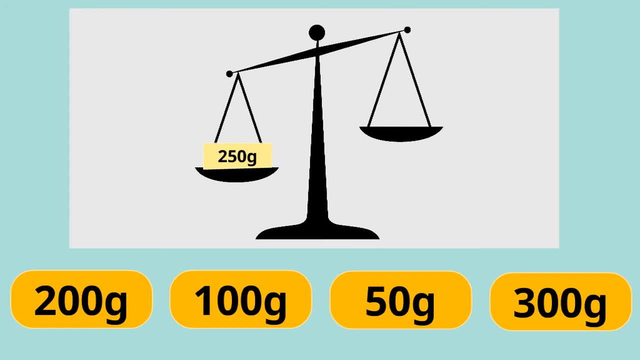 video and give it a try. Well, the two weights we would need are the 200 gram weight and the 50 gram weight. That will make the two sides equal. Well, the two weights we would need are the 200 gram weight and the 50 gram weight. That will make the two sides equal. 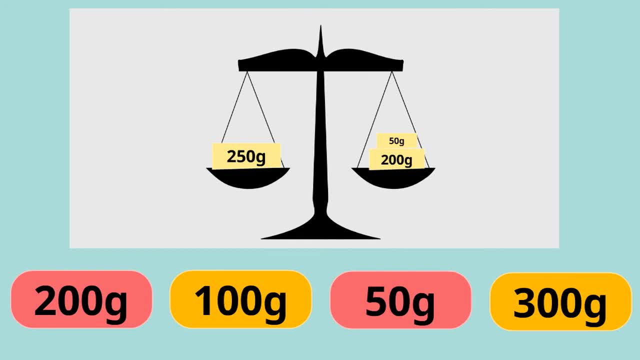 Well, the two weights we would need are the 200 gram weight and the 50 gram weight. That will make the two sides equal. Let's go for one last practice one, and this is probably the most difficult one so far, because you're gonna need more than one weight to balance this scale. 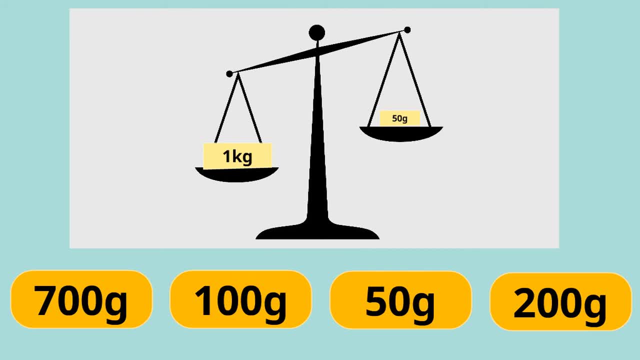 You can use any of the weights down below, but you must make sure both sides are equal to 1 kg. Can you pause the video and figure it out? Remember, there's a thousand grams in a kilogram. Did you get that one? It was quite hard. So we need the 700 gram, the 50 gram and the. 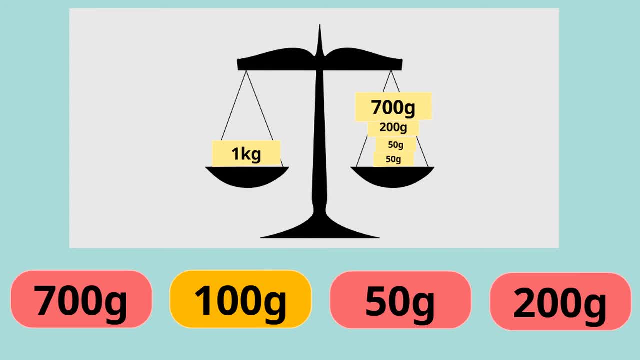 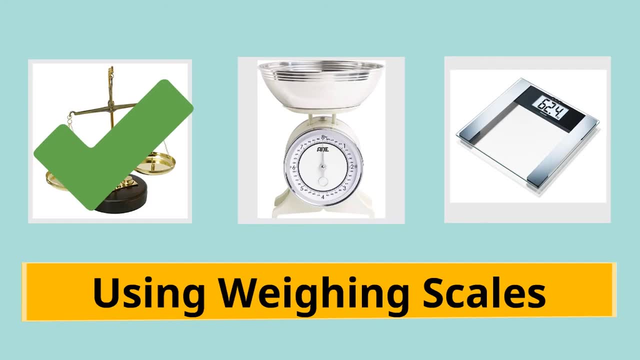 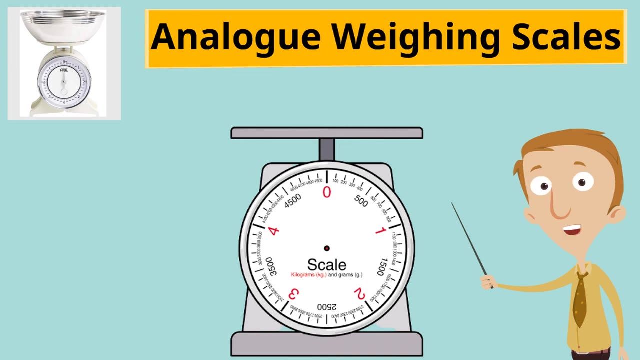 200 gram, That would make both sides equal to 1000 grams. Great, so now we know how to read off a balance scale. Let's have a look at analog scales next. The face of an analog scale is a little bit similar to the face of a clock. There are small lines and large lines. The small lines: 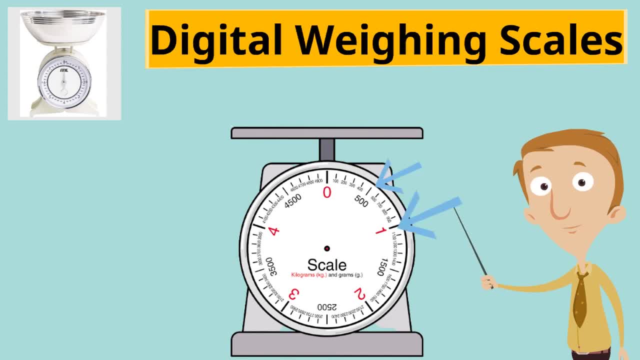 are the grams. The large lines are the kilograms. So this big one here is 1 kilogram and this 500 is 500 grams. Then we place an item on top of the weighing scales, The little red, and spins around to the correct weight and you just need. 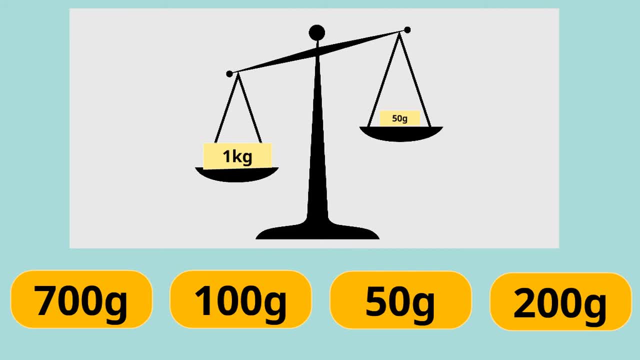 and figure it out. Remember, there's a thousand grams in a kilogram. Did you get that one? It was quite hard, So we need the 700 grams to make it equal. Let's try another one. Let's try another one. 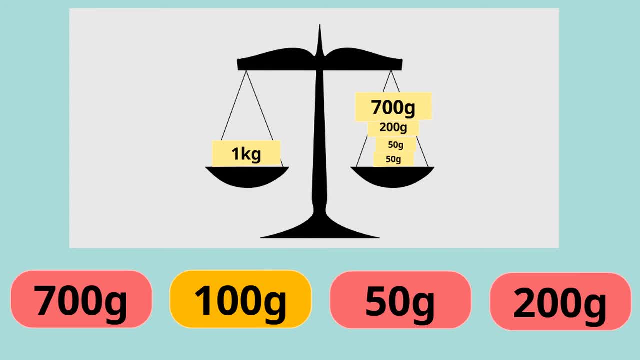 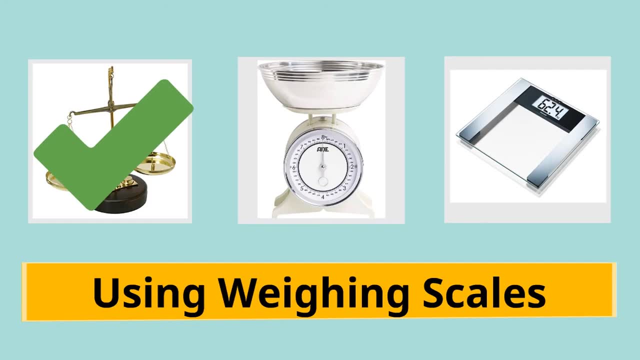 The 50 gram and the 200 gram. That would make both sides equal to 1,000 grams. Great, so now we know how to read off a balanced scale. Let's have a look at analog scales next. The face of an analog. 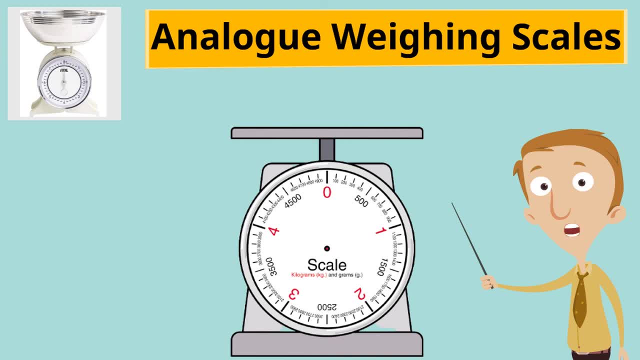 scale is a little bit similar to the face of a clock. There are small lines and large lines. The small lines are the grams, The large lines are the kilograms. So this big one here is 1 kilogram and this 500 is 500 grams. Then we place an item on top of the. 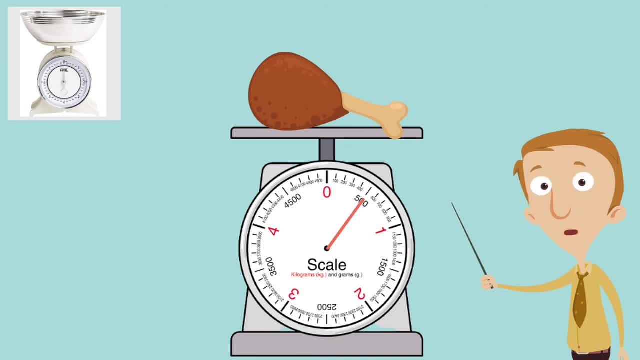 weighing scales, The little red and spins around to the correct weight, and you just need to read off which line it's closest to. So in this case, this delicious stick of chicken weighs 500 grams. Easy peasy. So let's do a few practice questions. 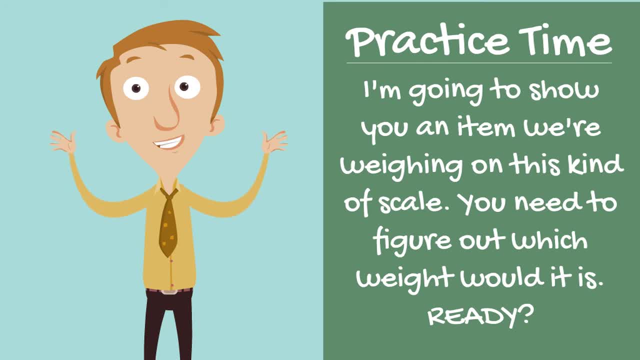 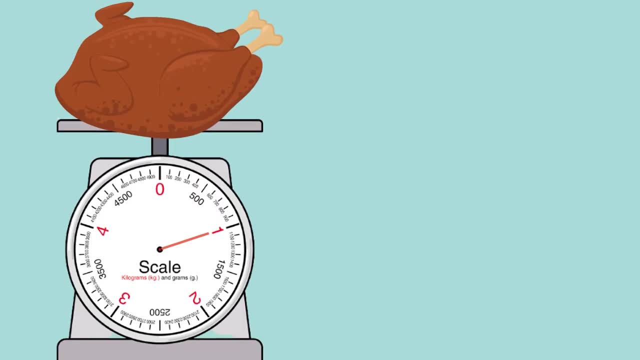 I'm gonna show you a weighing scales that has an item on it. What I want you to do is figure out what weight it is. You ready? Okay, here's your first item: How much does this delicious turkey weigh? Pause the video and write down your. 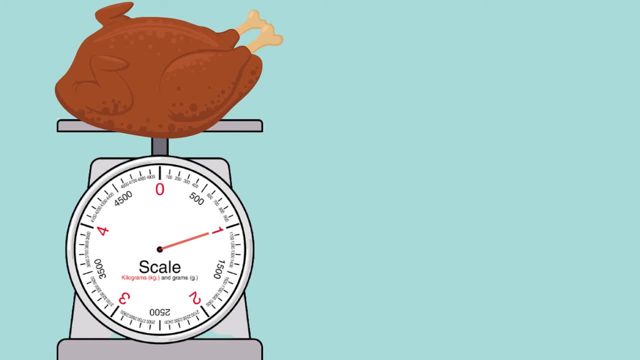 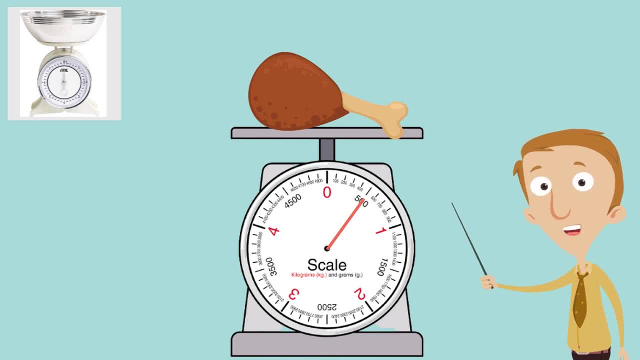 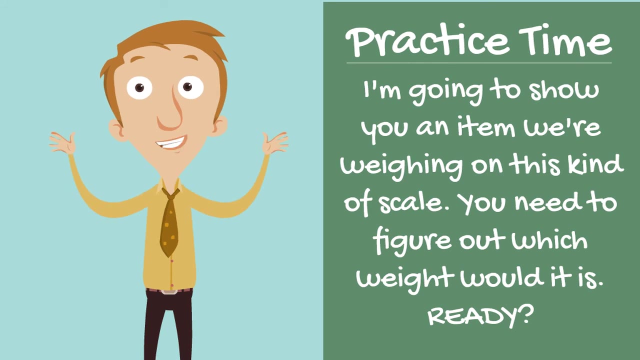 to read off which line it's closest to. So in this case, this delicious stick of chicken weighs 500 grams, Easy peasy. So let's do a few practice questions. I'm going to show you a weighing scales that has an item on it. What I want you to do is figure out what weight it is. 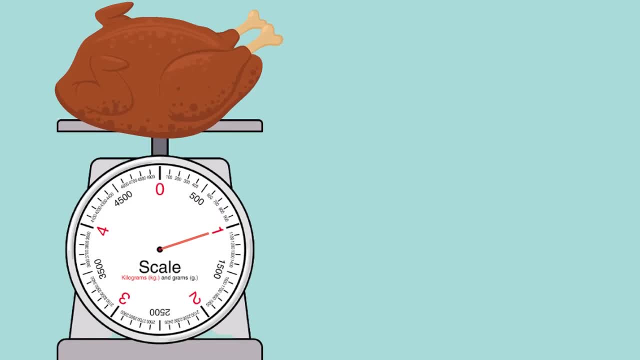 You ready? Okay, here's your first item. How much does this delicious turkey weigh? Pause the video and write down your answer. Well, it's at the first big line, so it weighs 1 kilogram. Next one: What about this also delicious looking burger? How much does this burger? 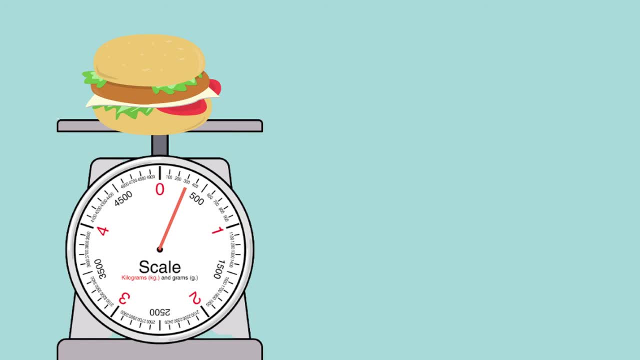 weigh? Pause the video and write down your answer. Well, this burger is at the third small line, so it weighs 300 grams. Next beautiful piece of food. Oh, it's a whole basket of food. How much does this picnic basket weigh? Pause the video and write down your answer. Well, 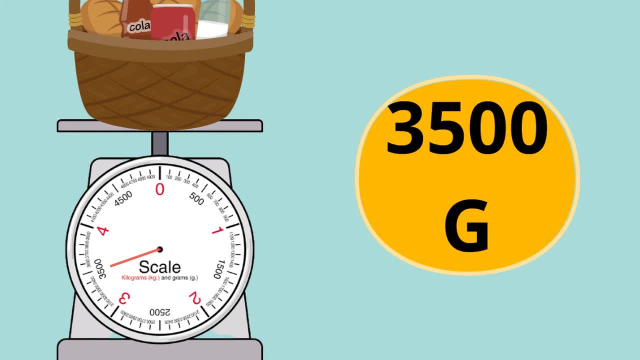 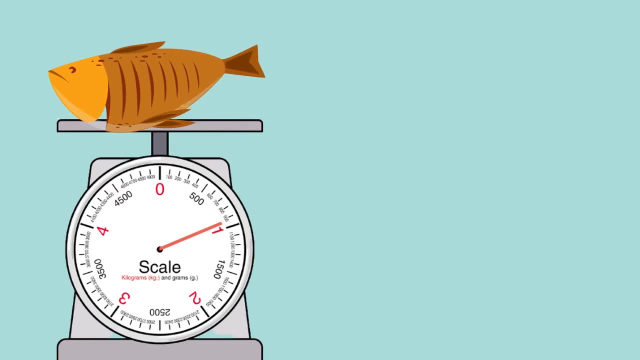 it's at the third small line, so it weighs 500 grams. What about this delicious duck? It's at the third small line, so it weighs 2 grams. Well, you can see that the red hand is pointing at 3500.. So that's 3500 grams, or three and a half kilos, and 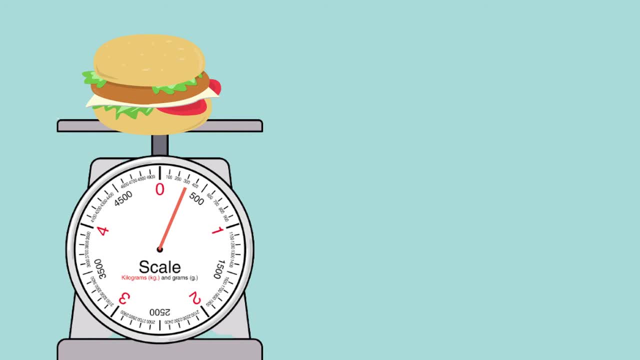 How much does this, How much does this? How much does this does this burger weigh? Pause the video and write down your answer. Well, this burger is at the third small line, so it weighs 300 grams. Next, beautiful piece of food: Oh, it's a whole basket. 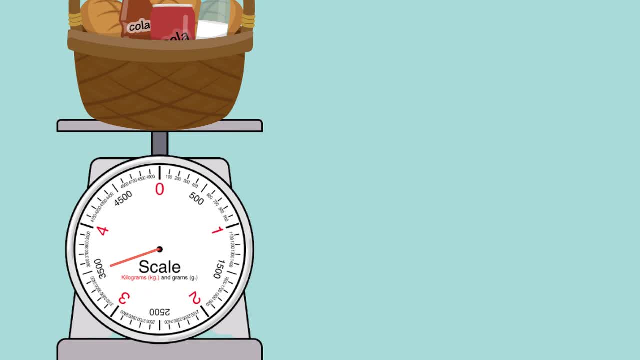 of food. How much does this picnic basket weigh? Pause the video and write down your answer. Well, you can see that the red hand is pointing at 3,500, so that's 3,500 grams, or three and a half kilos. And one last one: How about this not so delicious looking fish? How much does this fish? 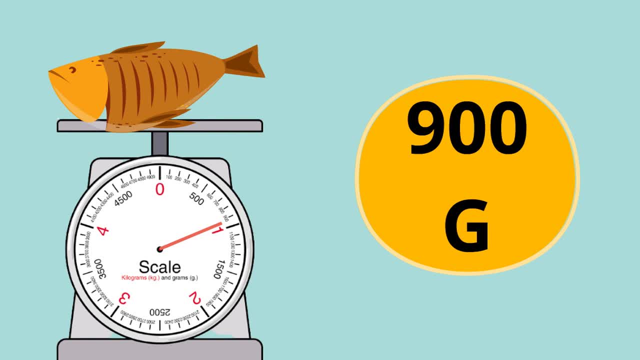 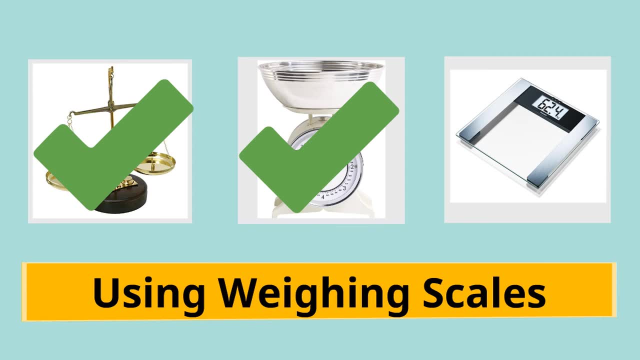 one last one. How about this not so delicious looking fish? How much does this fish weigh? Pause the video and write down your answer. read balance scales and we know how to use analog scales. The last one you'll be glad to hear. 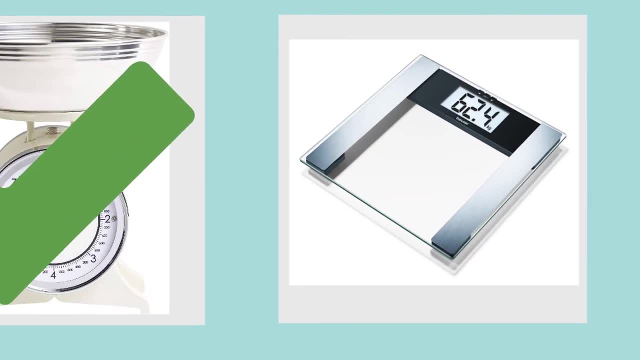 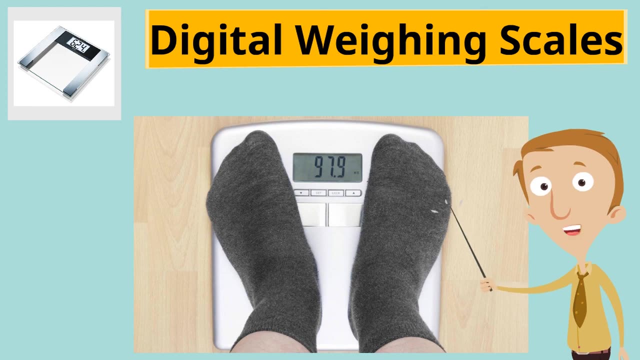 is the simplest one ever: a digital weighing scales. These weighing scales do all the hard work for you. As long as you've got batteries in, it can't really go wrong. You place the item you want to weigh on top of the scales and on the digital interface. here it will tell you how much. 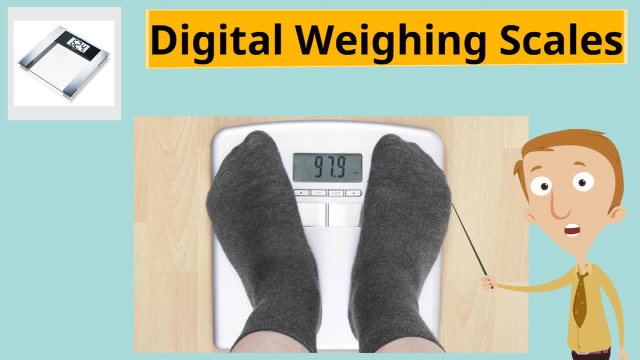 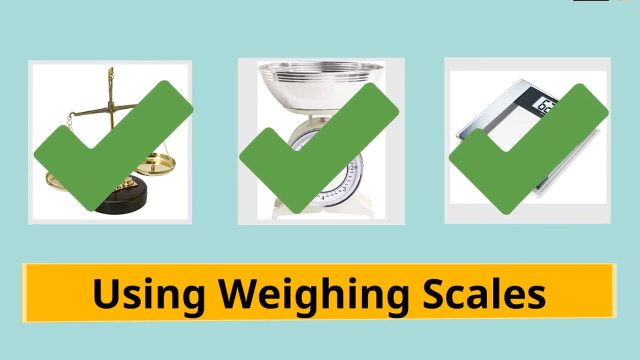 it weighs in grams and kilograms. The only thing you need to be careful of when you're using a digital weighing scales is to make sure that it is in the kilogram and gram setting. Sometimes it might accidentally go into different settings And that's it. Three for three Balance scales.